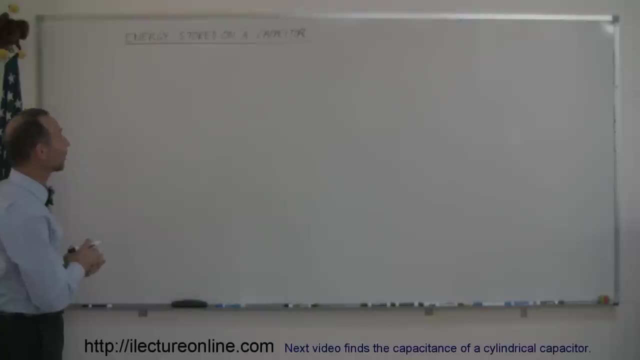 Welcome to iLecture Online, and here's the next topic dealing with capacitors and, in particular, how much energy is stored on a capacitor. and, as we saw in previous chapters, when you push charges across a potential difference, you create energy. actually, you store energy into a device, and so a capacitor is kind of 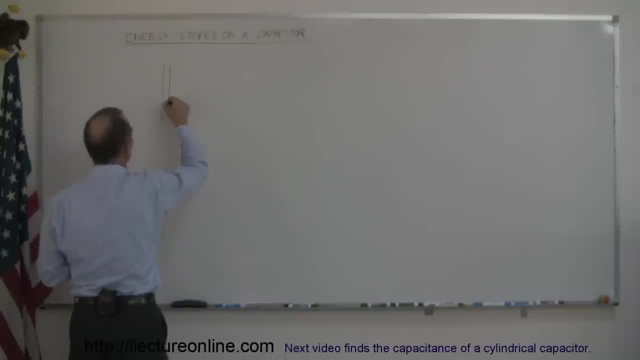 like that. so imagine that you have a capacitor with two parallel capacitor plates and you connect that to a battery or a voltage source like that. so voltage source equal to V, Let's say the capacitance has capacitors C, and let's put a switch in there so we can kind of go like this: The switch currently is: 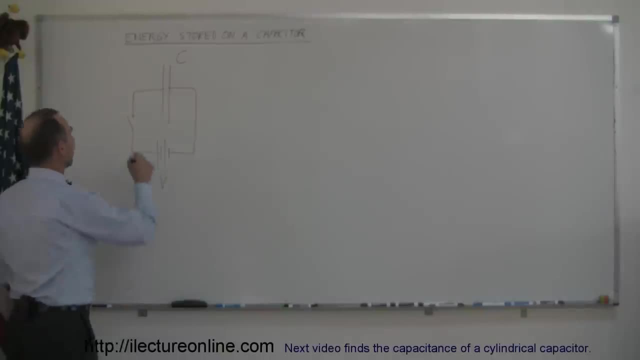 open, which means there's no charges flowing to the capacitor. and at the moment when we close the switch, charges coming from the positive end of the battery will flow through the circuit here and start depositing themselves onto the capacitor plates, and slowly- well depends, maybe fast. 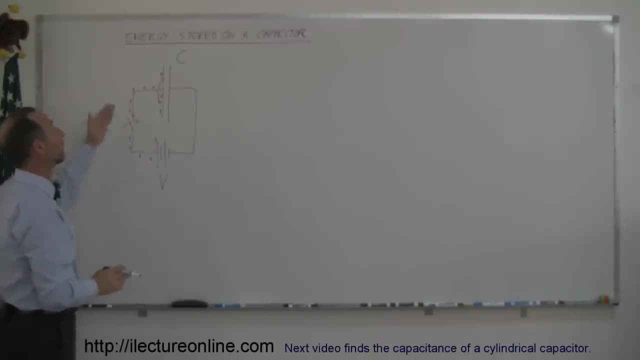 depends what, what the circuit is made out of. maybe very fast we'll start putting charges onto the capacitor plate, pushing positive charges away on the other side, making the other side of plate negative, as these positive charges flow back to the negative end of the battery. so by doing that it has the 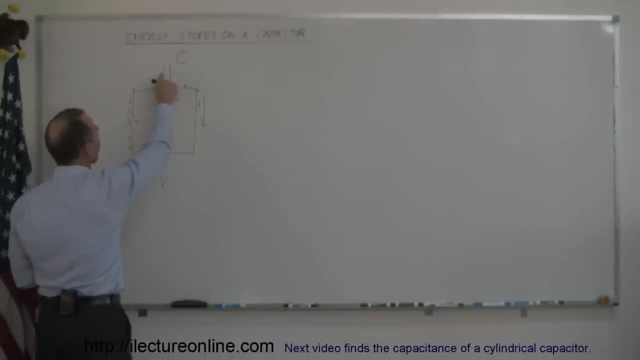 effect of moving. every time you put a charge on the side of a capacitor plate, it has the same effect as if you were to take a charge and move it across the gap between the plates. it's like pushing the the charge across. so if you remember when we did that before, that the work done to move charges across a gap was 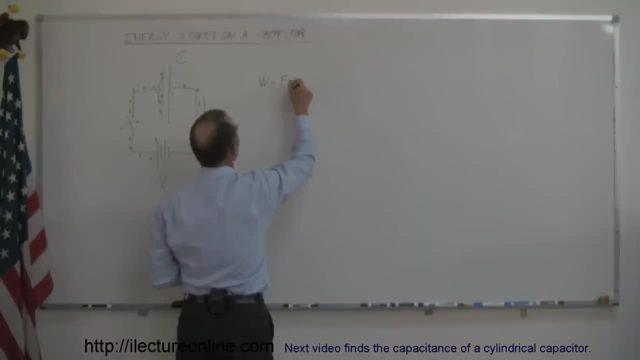 equal to the force that they were experienced, times, the times, the distance that they traveled. and that would be equal to the force, but in electric field is equal to E times Q, so it would be E times Q times D, and E times D is the potential difference, so we can write this as E times D times Q. 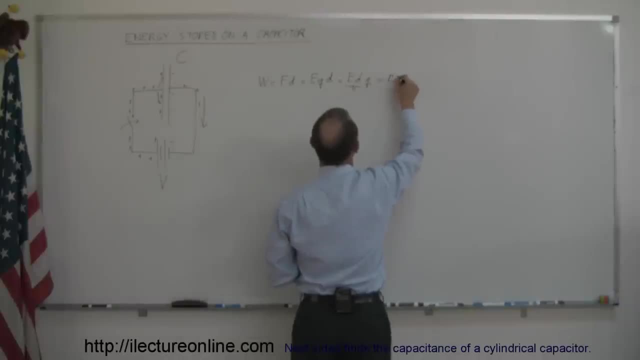 and this here is the same as the potential difference between the plates times Q. so the work to the work done to put each charge on the capacitor plate equals the potential difference at that moment in time, times the charge that you just placed there. so you can imagine when you put the first charge there and 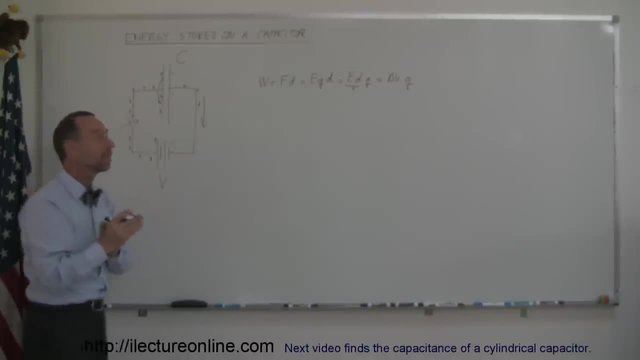 there's not not yet any potential difference between the plates. to put the first charge there, it takes zero joules. it takes zero joules, it takes zero joules, no work at all. but to put the last one there, when you place the last one there, the capacitor is already fully charged and the potential difference across the 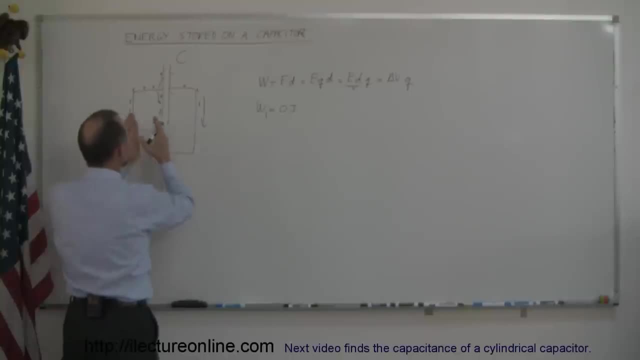 plates is essentially the same as the potential difference across the battery, equal to V. so to the work done to put the last one there is equal to the change in potential difference, or V times the charge on there. so how much energy or how much work do you think it takes? 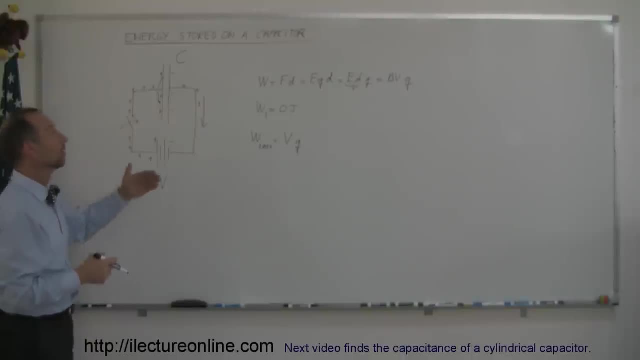 to put the middle one there. let's say you put a thousand of them on there, the first one would take zero joules, the last one would take this many joules and the one in the middle, halfway through, would take half that much so the work done to. 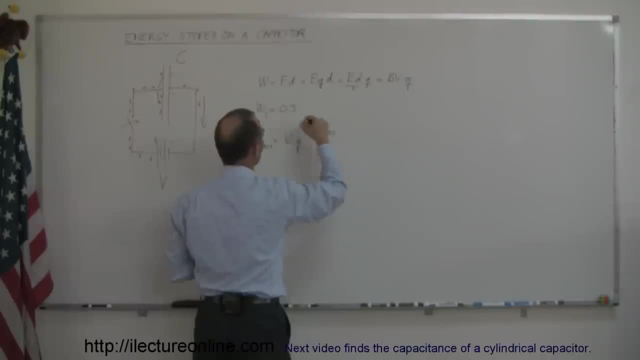 put the middle one in, there would be, on the average of the two or one half V times Q. so it then follows by this logic then if you put all of the charge and aren't on there, so that Q is simply the sum of all the little Q's, one at a time. 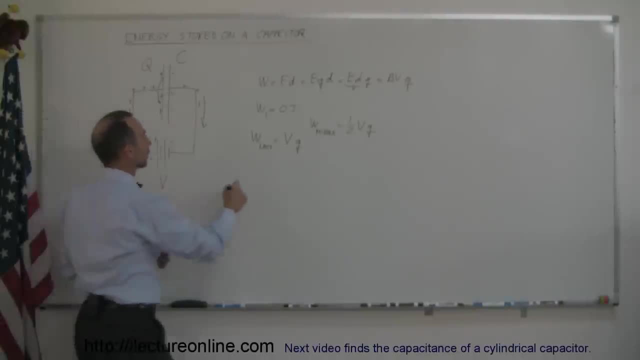 Q is a total charge of all of them put together, that the work done to put the total amount of charge on there would then be equal to one half the voltage times Q, and that would then be the work done to put all of them on there all. 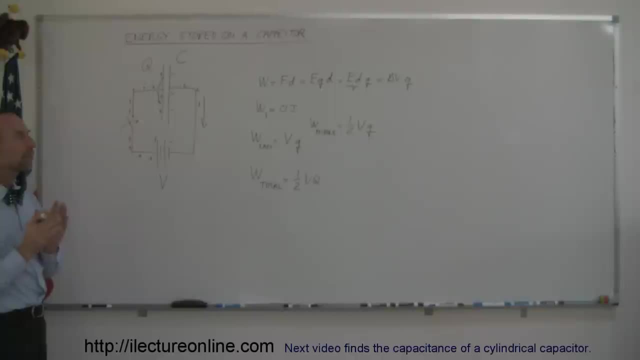 right now, going back to the definition of capacitance, we can say that the capacitance is simply equal to the ratio of the charge that you put on the capacitor divided by the voltage you put on there. so we could potentially replace Q by C times V, or we could potentially replace: 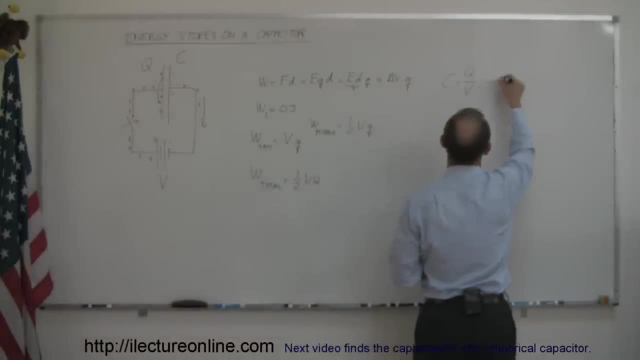 V by Q over C. so here I can take this equation and say that Q is equal to C times V. or I can say that V is equal to Q divided by C. so we can take those two equivalents of Q and V, plug them in here so we can say that the work total can. 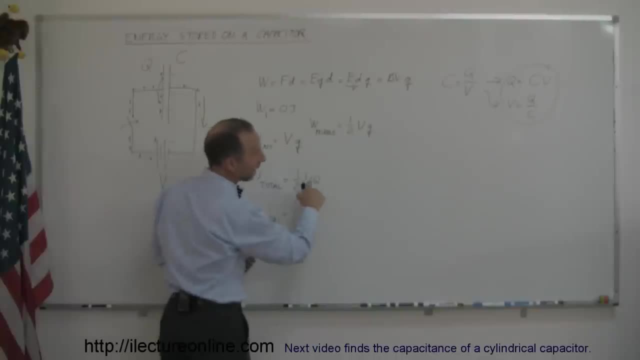 also be expressed as one half times instead of V. I can write Q over C, so Q over C times Q, which is equal to one half Q squared over C. or I can say that the work total is equal to, and I can take the original equation and replace Q by C. 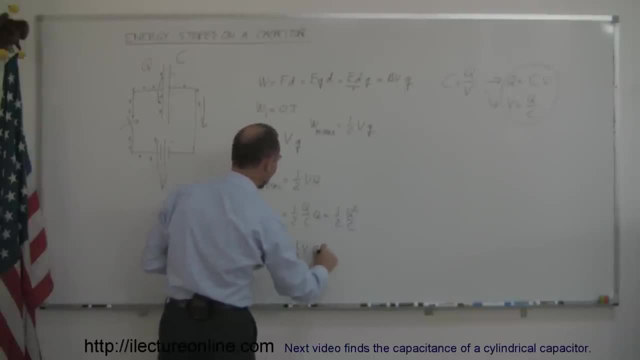 times V. so that would be one half V times C times V, or one half V squared C. so these are the three ways in which you can calculate or describe the total work done or the total energy stored on a capacitor when it's filled with charge. and then, of course, if they tell you, for example, that you have a 20 volt battery. 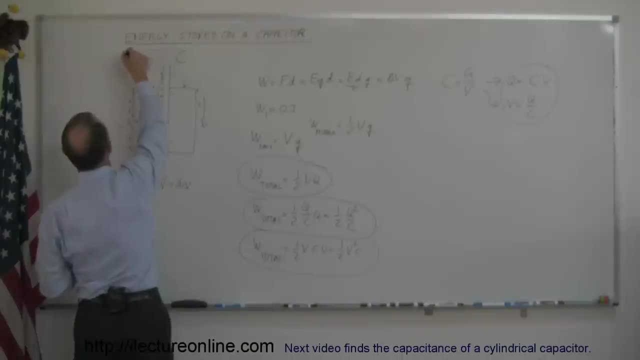 and let's say that you have 50 micro coulombs word of charge on the capacitor, then if you say, well, how much energy is stored in the capacitors of the energy stored is equal to the work done to to put all that charge on there. 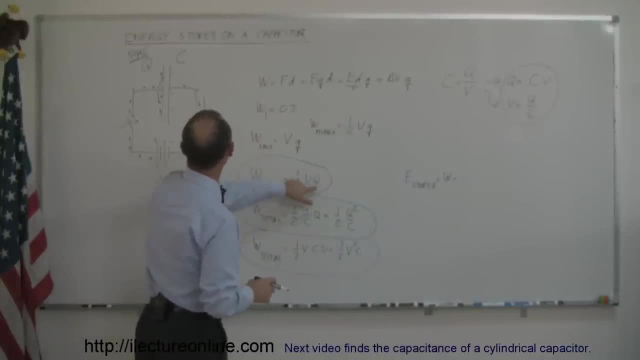 the work done can be described as one half V times Q. we have the voltage, we have the charge, so we say that's equal to one half V times Q, which is equal to one half times the voltage. the voltage is 20 volts and the charge Q is 50 times. 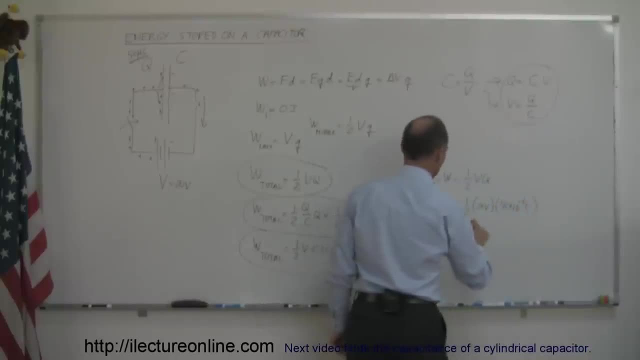 10 to the minus 6 coulombs, so that would be equal to one half times 20 times 50 of the thousand times 10 to the minus 6. that would be 1 times 10 to the minus 3, and that would be joules voltage times. coulombs is joules and. 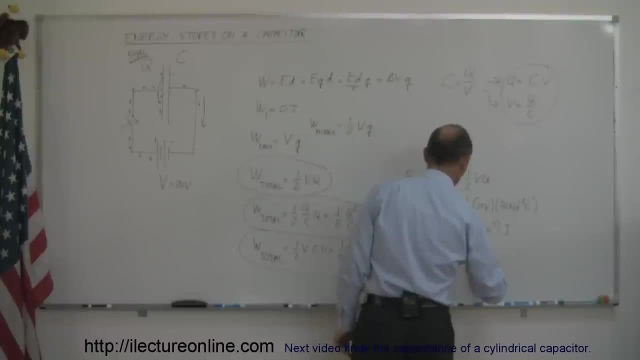 one half that. that would be equal to 0.5 times 10, to the minus 3 joules, and that would be the total energy on the capacitor. this particular capacitor is the potential difference of 20 volts and the charge on the capacitor is 50. 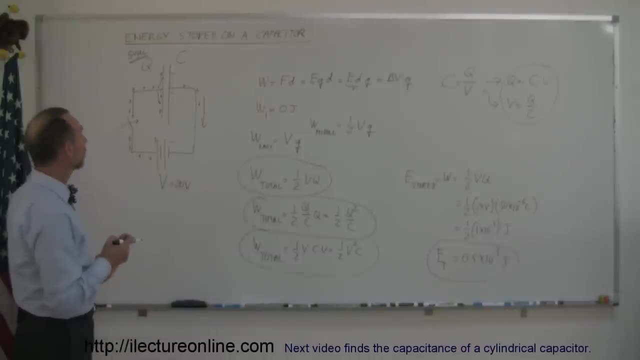 micro coulombs. and just for let's see if we remember this, how big is the capacitor? what is the capacitance of a capacitor that will sort 50 micro coulombs of charge when there's 20 volts applied? well then, we go back to. 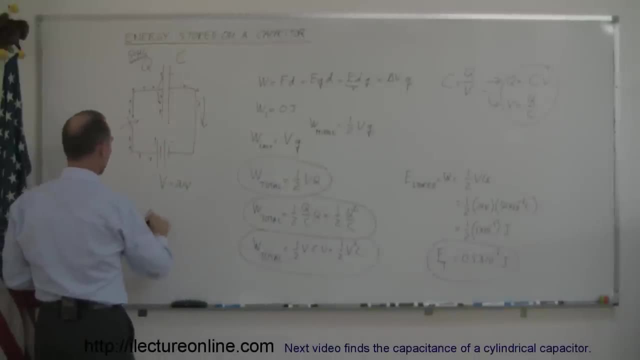 that equation. right there, we can say that capacitance is equal to the charge divided by the voltage, which is equal to 50 micro coulombs, divided by 20 volts, which is equal to 2.5 micro farads. so in this case we're dealing with a 2.5. 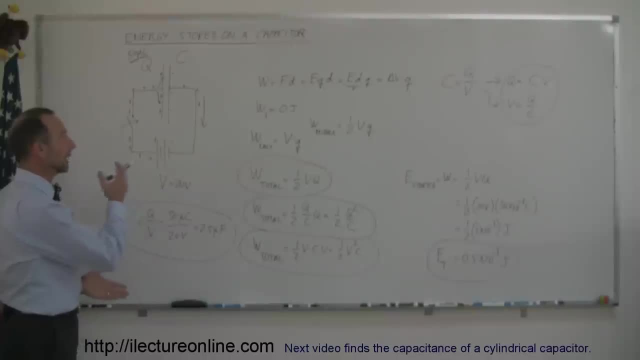 micro farad capacitor and that's how you work with the energy stored in the capacitor when you fill it full of charge. all right, hopefully that helps. a little side topic, but you never know, you probably were into some homework problems just like it on your homework. all right, good luck with your work. with ease.